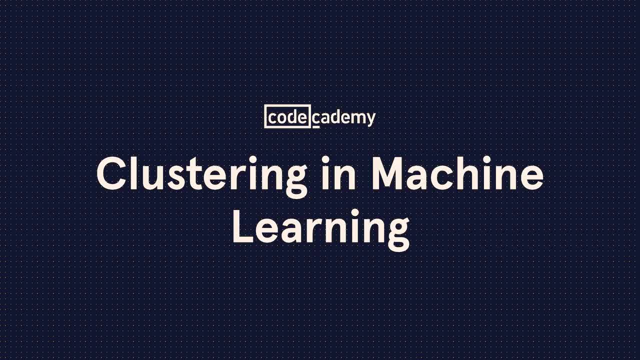 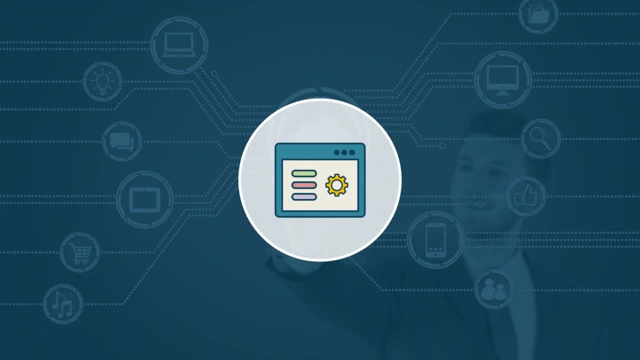 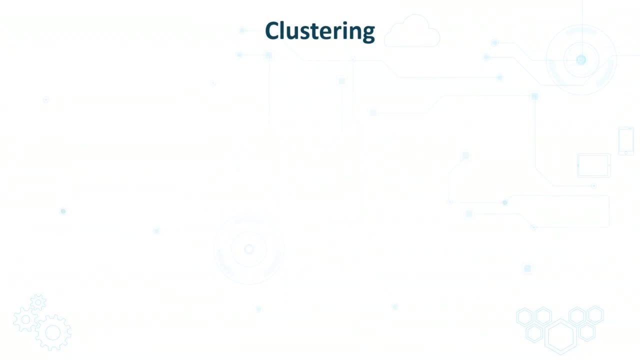 We will now take a closer look at one of the techniques used in unsupervised learning, which is referred to as clustering. So what exactly is clustering? This is a technique where your data is divided into a number of logical groups. This grouping is done based on the characteristics of 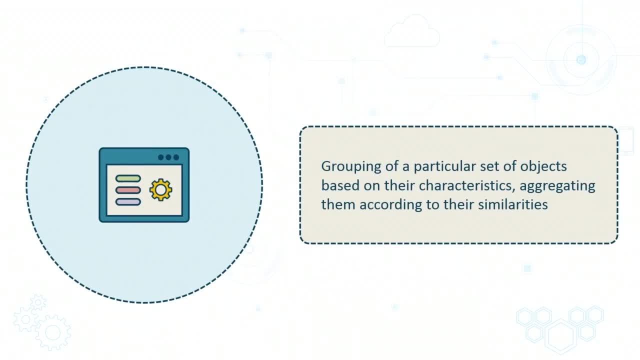 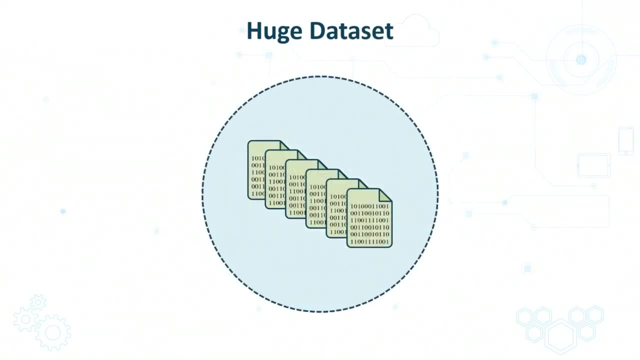 the data and all of the data within a particular cluster will have certain similarities. To understand this, consider that you have a huge data set where you have millions of data points and there are no labels for you to work with Before you use the data for anything. 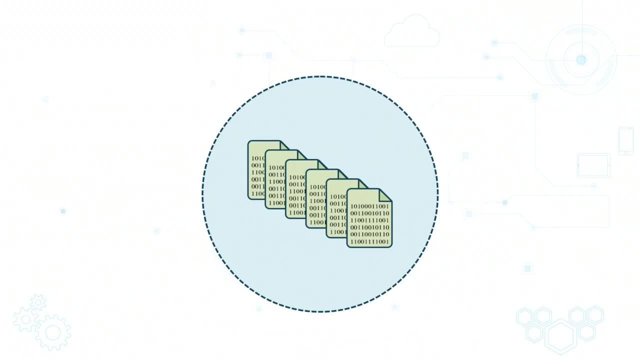 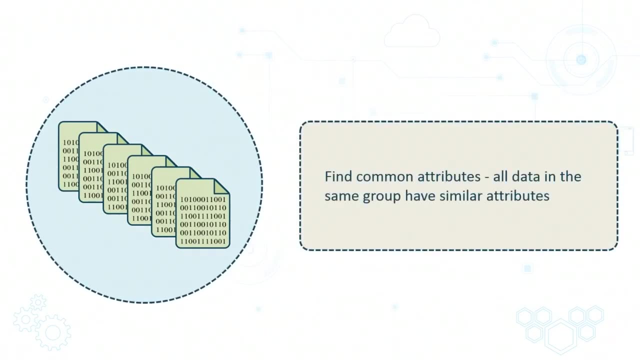 you want to see if there are any patterns which can help you identify groups in your data. For that you can make use of a clustering algorithm, and these will examine all of the attributes in your data set and will be able to determine that there are several data points. 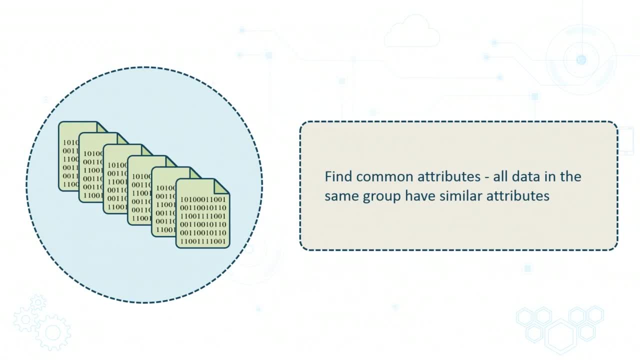 which share similar attributes or characteristics. Based on the similarities, a number of different groups may be formed in your data set, and each of these groups will form a cluster of data points. So the task of a clustering algorithm is to examine the data which is presented to it. 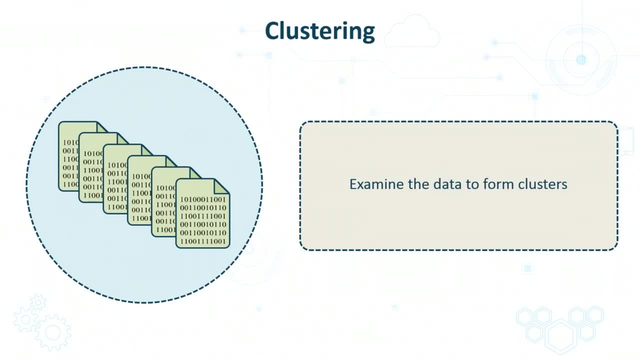 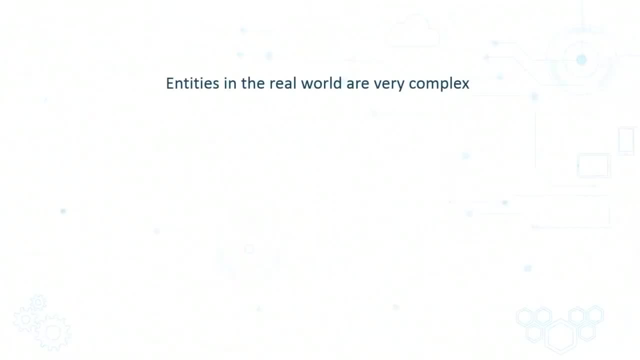 and then break it up into a number of logical clusters. All the data points within a cluster will have far more in common than with points outside the cluster. So why exactly would you want to employ the technique of clustering? Well, consider that entities in the real world are, in fact, very complex and may not be very easy to categorize. 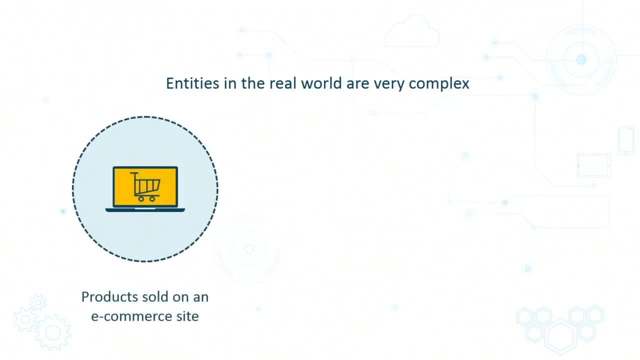 For example, you may have a lot of data about the products which are sold on an e-commerce site, but how many different categories should you divide them into and what exactly should those categories be? You're faced with similar questions when categorizing the users. 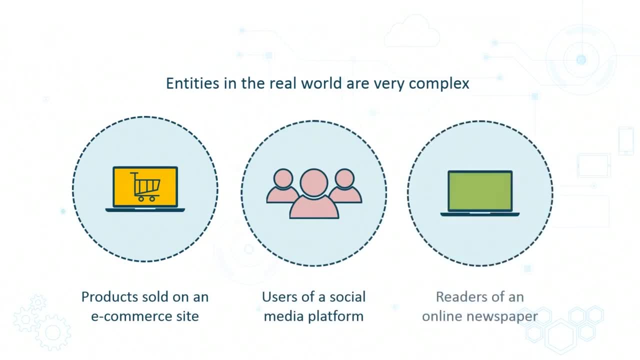 who are on a social media platform, or even in the case of readers of an online newspaper. Do you classify people by their age, their gender, their geographical location? And if you do all of the above for geographical location, then what exactly is the definition of a single location? 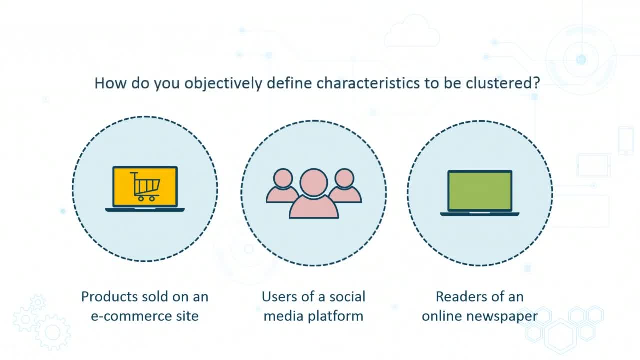 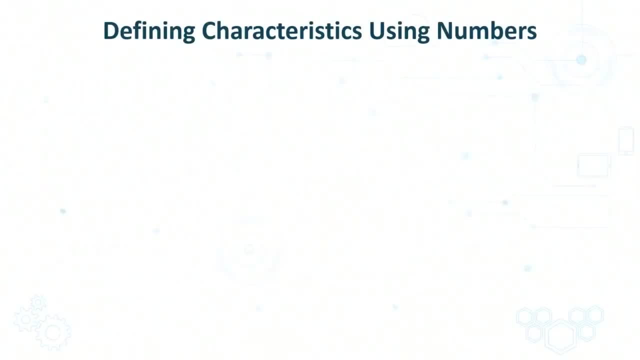 Do you divide people by state, by city or by neighborhood? So there is clearly no way to objectively divide your data into groups. This is where clustering comes into the picture, but before you can apply it, you will need to ensure that the defining characteristics of 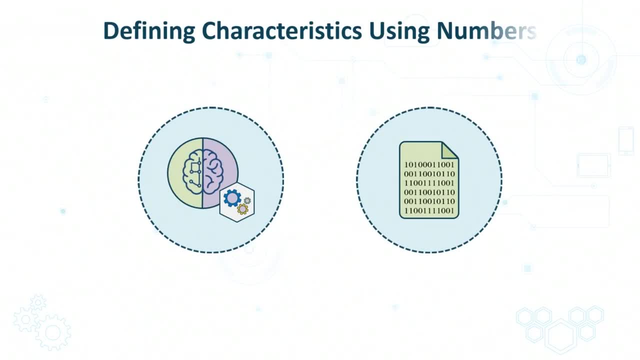 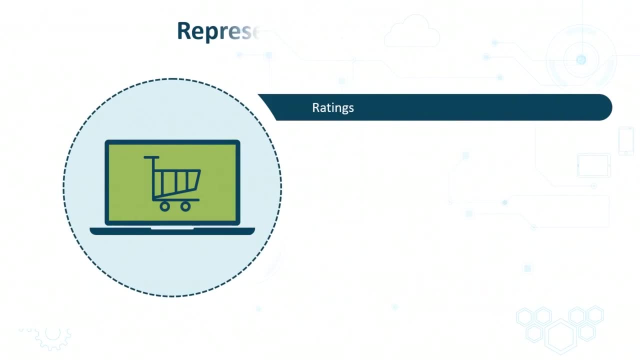 each of your data points are represented using numbers. For example, in the case of products, one of the attributes of the data can be a rating, which is given to the data point. So, for example, a rating can be given to the product by the users. They can also be an overall review sentiment. So 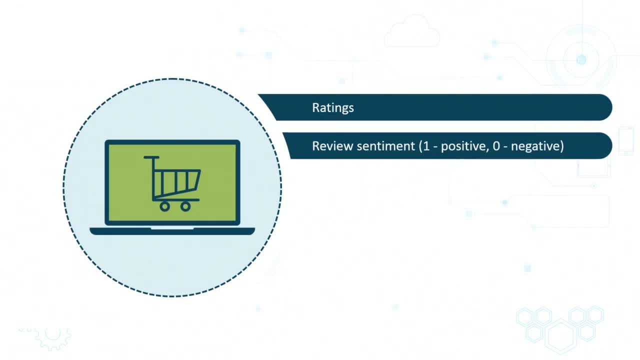 for all of the reviews made for the product, you may come up with an aggregate sentiment score, which could range somewhere between 0 and 1.. The attributes, in fact, need not be entirely numeric, but could be categorical, with numeric labels representing each of the categories. 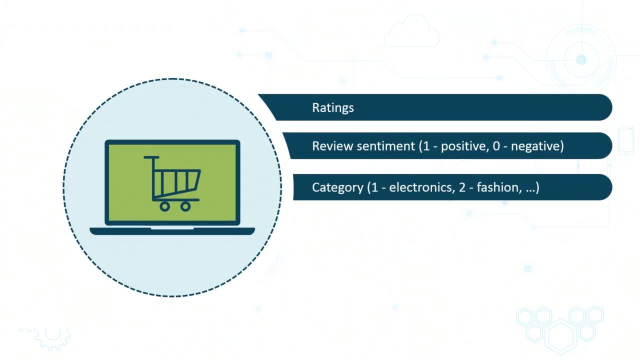 For example, the number 1 could represent electronic products and number 2 for some fashion accessory. Some other attributes for a product could include the dimension, such as the size, the weight and so on. You may even have a color for the product, and this again. 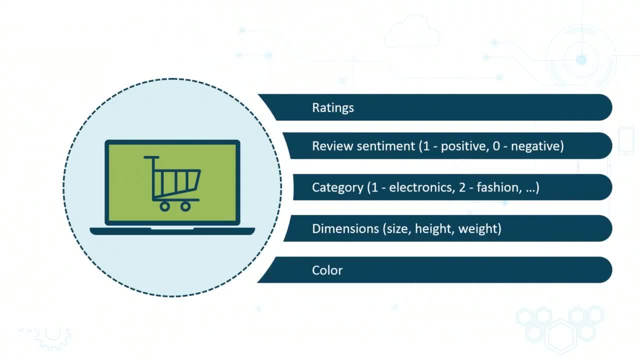 because it's a categorical value, will need to be represented by some numeric label. So, for fields such as the product category and the color, these are some of the predefined categories you come up with, but your clustering algorithm may help you identify certain other. 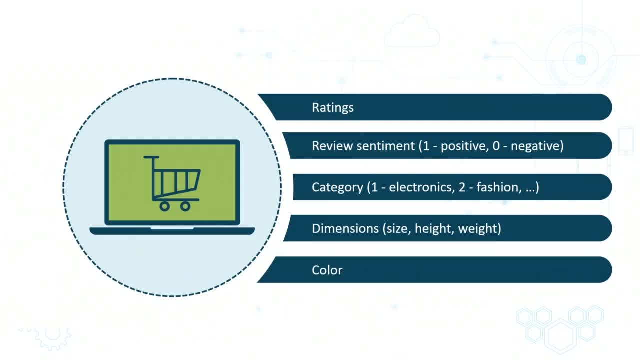 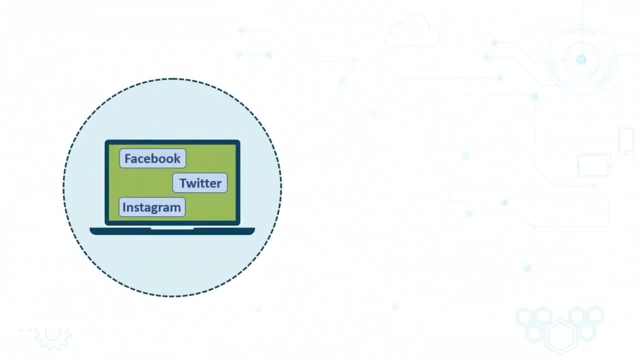 categories, For example, highly rated electronic items, which are available in blue. Moving along now to the defining characteristics of users when it comes to data points. So on the social media platform, you may have some kind of rating for the posts made by the user. 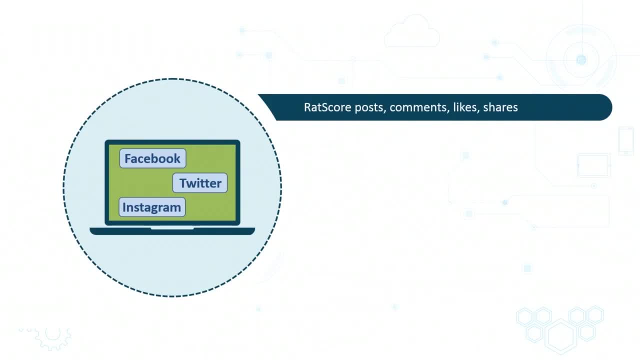 as well as the comments, likes and shares. You may even have some kind of categorical labels for each of their posts, and this could be by the topic of that post itself. You may rate each user or reader by their activity on the platform, So 100 can represent a highly 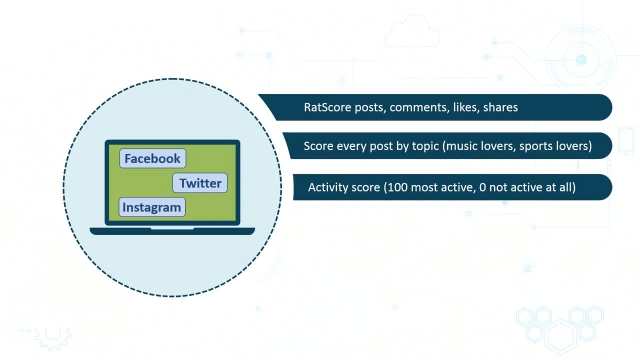 active user and 0 if they are not active at all. In the case of social media, you may rate each user based on data points and rate them based on the activity of the user. So, for example, if I'm user by the number of connections which they have, and you may also give a score for. 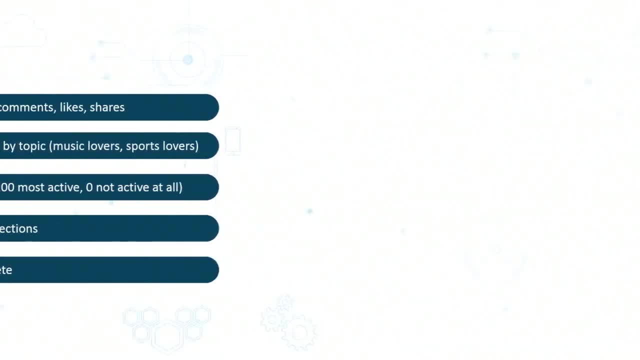 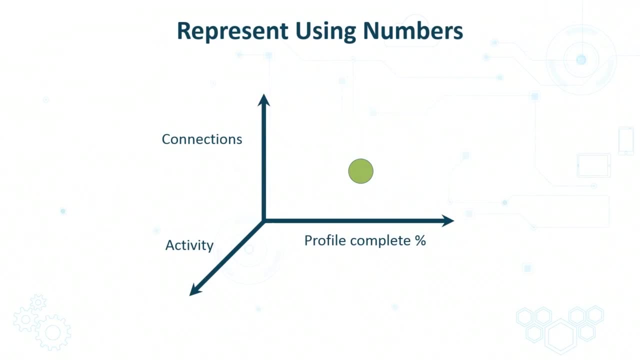 each user depending on how complete their profile is. So, sticking with the example of users on a social media platform based on the factors such as connections, activity and profile completeness, you can represent each user by a point on a three-dimensional plot such as this one: 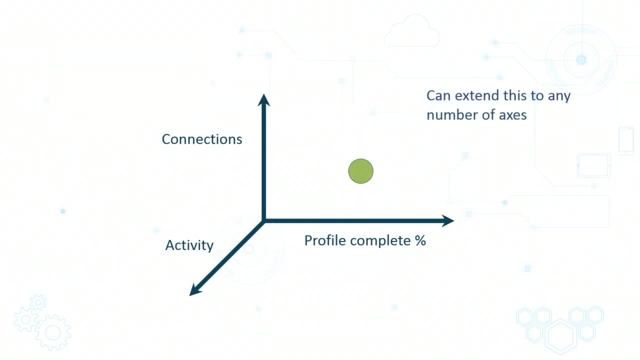 Rather than just considering three attributes, you can extend this to n attributes, where you'll have an n-dimensional hyperplane on which you will represent your users as points. Once each user is represented as a point on this hyperplane, then there will be number of points which happen to be close to each other in terms. 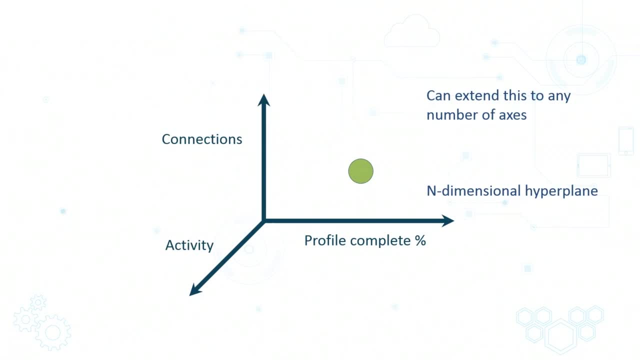 of overall distance. So there may be one group of users who are very highly active but also have very few connections. As you can imagine, there is likely to be a cluster where the profile completeness is close to zero, as is the activity and probably the connections as well. 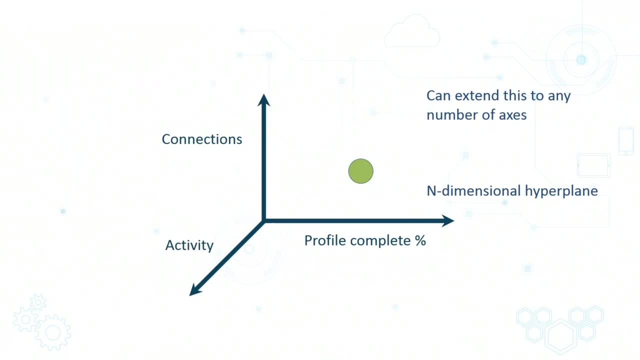 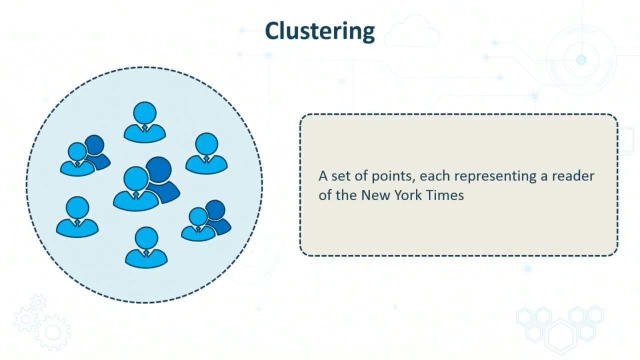 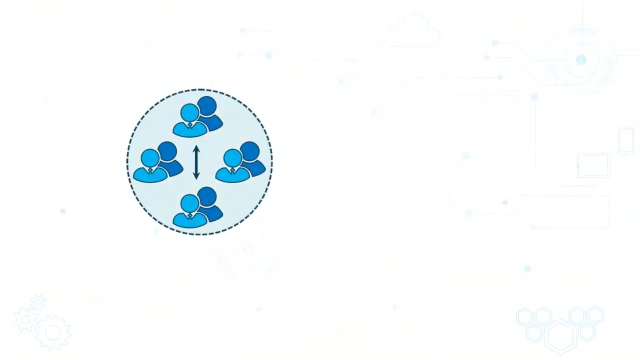 It is these kind of clusters which a clustering algorithm will help you find. Moving to another example, consider that you have plotted on an n-dimensional plane all the readers of a newspaper such as the New York Times. Well, if you implement some kind of clustering algorithm on these points, 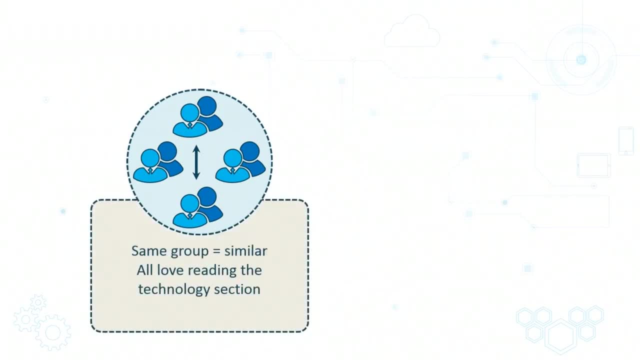 you may discover that one cluster represents users who spend a lot of time in the technology section of the newspaper, So that is one common attribute for all the members in one cluster. On the other hand, there will be different clusters and this may represent readers. 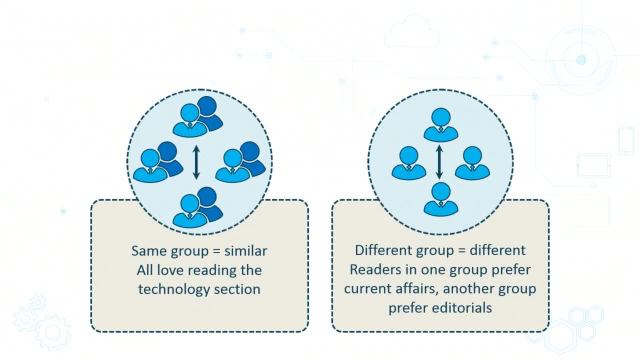 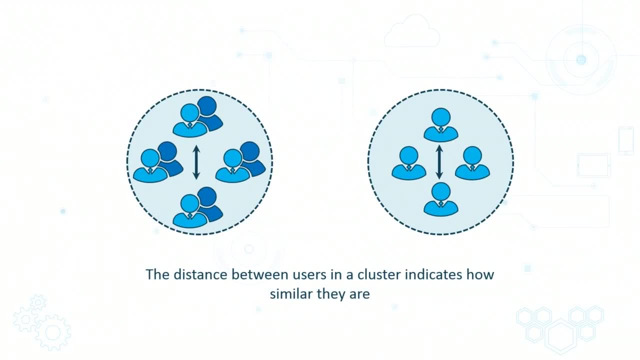 in different sections of the paper, such as current affairs or sports. So when you examine the users within a particular cluster, the distance between the users is an indication of how similar they are. So if you have one cluster where most of the readers read articles from the 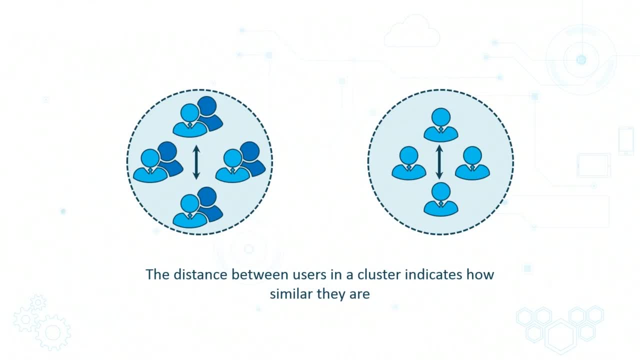 technology section, then those points which are close to each other may represent users who read multiple technology articles in a single day, Whereas you may have other points within the same cluster representing users who read technology articles just once a week. When dividing any data set into a number of clusters, the goal of the clustering 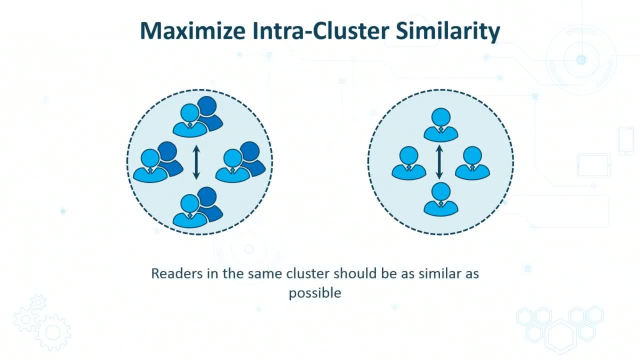 algorithm is to ensure that all of the data points within the same cluster should be as similar as possible. This may involve creating clusters based on multiple attributes rather than just a single one. So maximizing intra-cluster similarity is one of the goals of clustering, the other one being to minimize inter-cluster similarity. 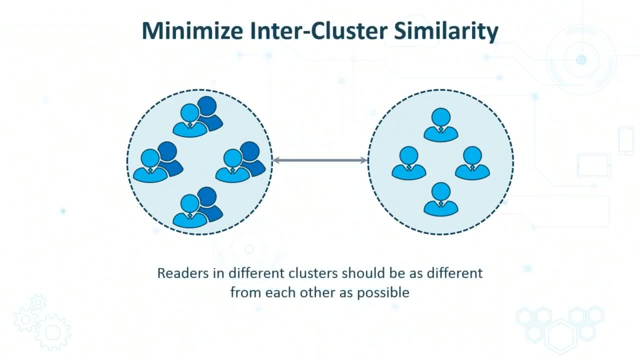 So all of the data points which are in different clusters should be as far apart as possible. This is where the number of clusters your data will be split into comes into the picture. Create too few clusters, then you may minimize the similarity between different clusters.